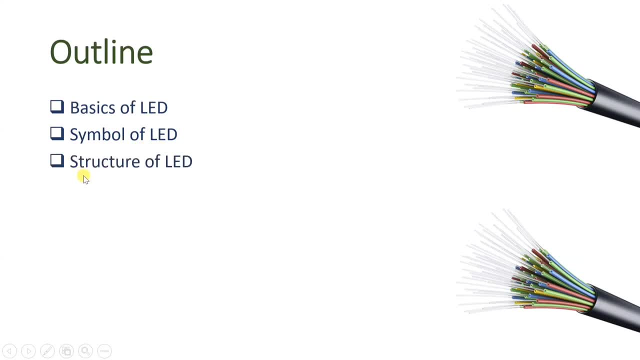 symbol of light emitting diode. Then, after I'll explain you structure of light emitting diode, Then we will see working of light emitting diode. Then I'll show you some material which is used to make light-emitting diode with different colors of LED, And at the end we 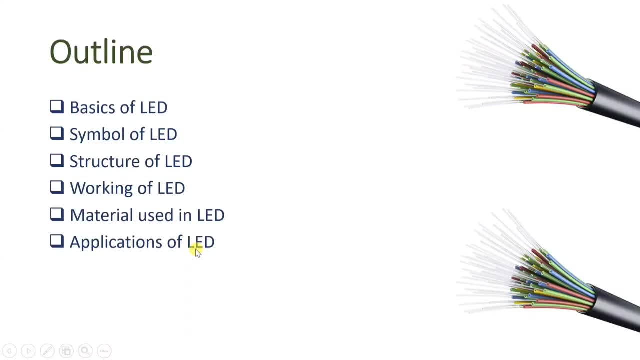 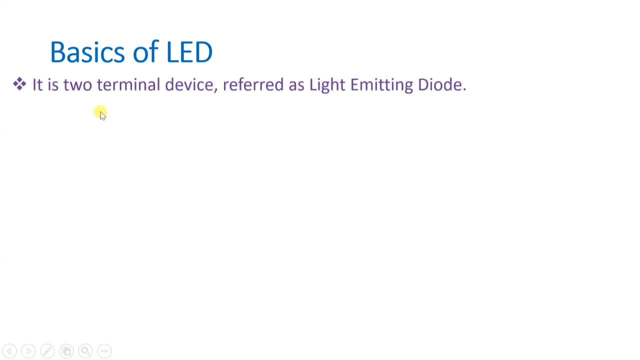 will see applications of light emitting diode. So let us begin this session with first agenda, that is, basics of light-emitting diode. So it is two terminal device and it is even referred as LED. LED stands for light, stands for emitting, and D stands for diode, so it is light emitting diode in. 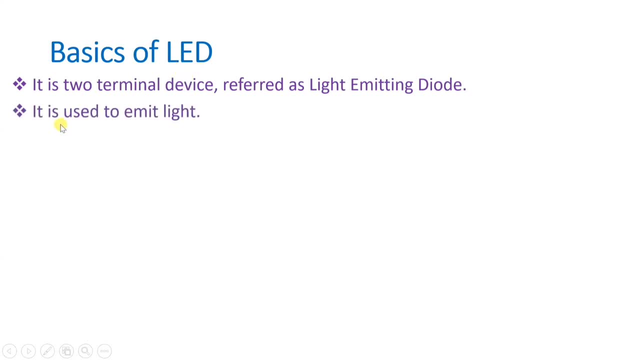 short, it is LED. it is used to emit light and its working principle is: it converts electrical signal into light signal. so usually in optical fiber communication we use LED to translate electrical signal into light signal and we pass that signal through optical cable. when we talk about LED, we use that. 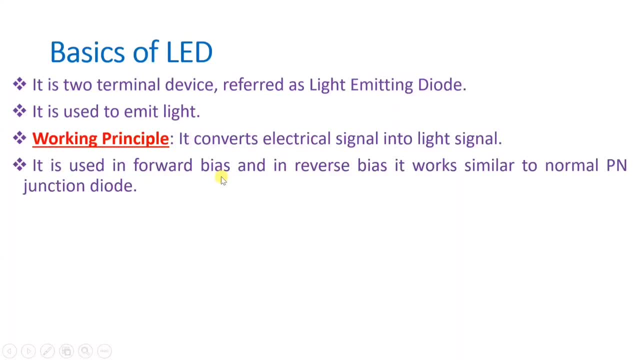 in forward bias. when LED is in forward bias it emits light and in reverse bias it works similar to normal p-n junction diode. so LED is used in forward bias and it's in reverse bias. it's working is similar to normal p-n junction diode. so 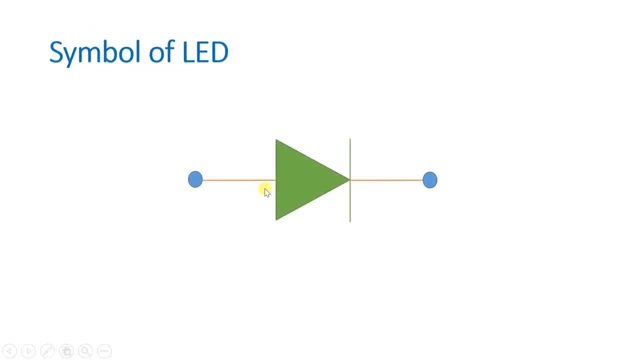 let us see the symbol first. if you observe symbol of LED, then that is almost identical to symbol of diode. you can see. but additionally here there are two arrows, which indicates this is a symbol of LED. so these two arrows plus symbol of diode is a symbol of LED and this 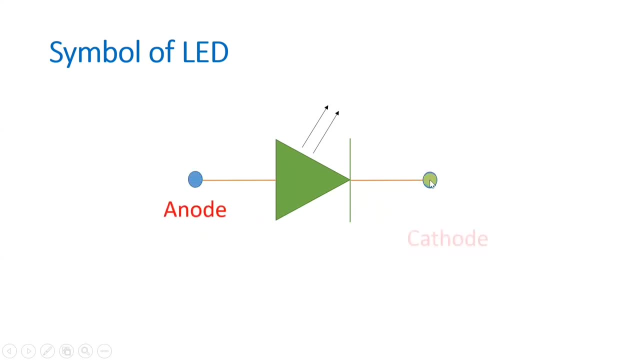 terminal that is anode terminal and this terminal that is cathode terminal. so this is what symbol of light emitting diode. now let us see the structure of light emitting diode. so this is a base which is there with light emitting diode structure, and here you can see there are two terminals: this bigger terminal, that 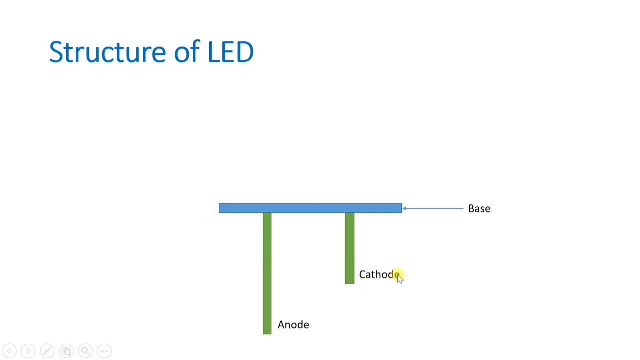 is anode terminal and this smaller terminal that is cathode terminal. when you observe physical structure of LED, then you will be finding there are two terminals: bigger one is anode and smaller one is cathode. this anode terminal is connected with p-type material and this cathode terminal. 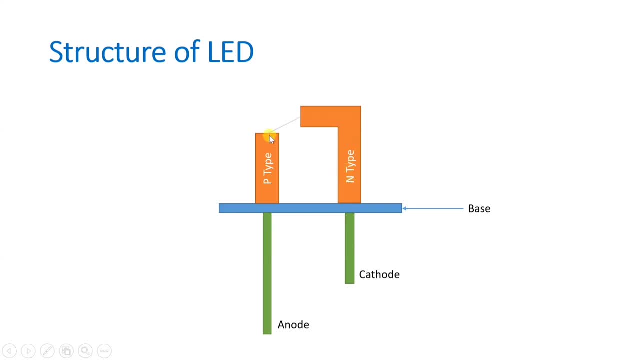 that is connected with n-type material and there is a contact in between these two, so that that is what we are having it to have: a radiation of light. so when you connect this LED in forward bias, there will be a generation of light at this contact and this light will get emitted out. if you have this cover, which 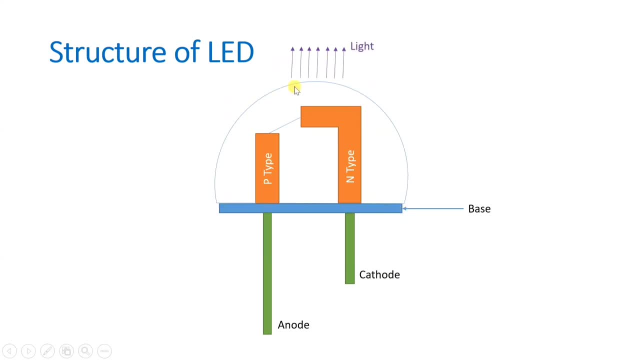 is transparent one, so we should be having cover that should be transparent cover so that this light can go outside. so this is what the basic structure which we have with LED. now let us see that structure internally and that gives you insight like how this LED functions. so, as I have told you, there is p-type. 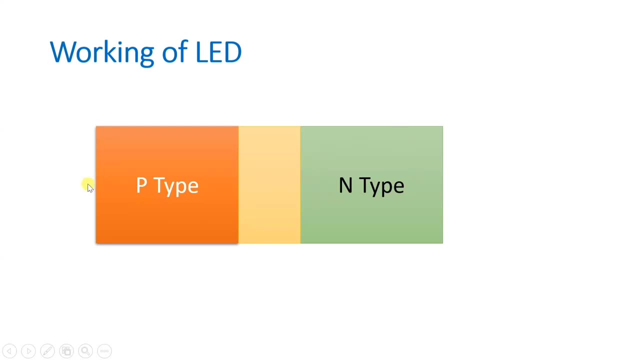 material and n-type material. p-type material is there at the side of anode and n-type material that is there at the side of cathode. p-type material is having holes as a majority carrier and n-type materials is having electrons as a majority carrier and at the junction there will be space, charge region or one. 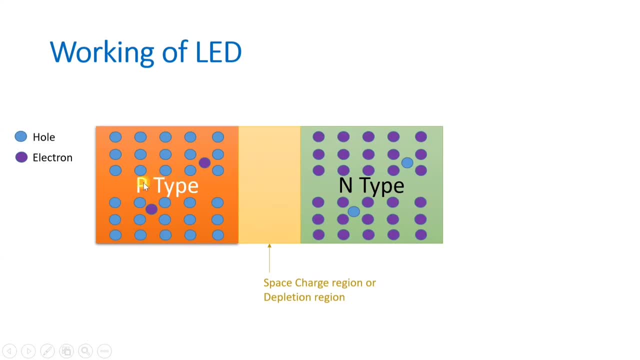 can say depletion region- now see towards p-type region means at this side there are holes and those holes are getting combined with electrons of n-type material. so these holes are accepted electrons and as that is accepting electrons, that is generating negative ions at the side of p-type material at junction and electrons are there with 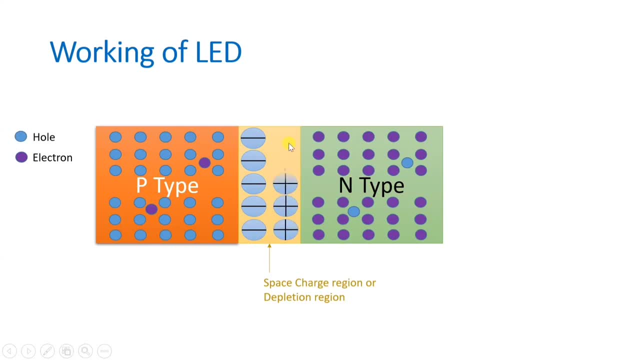 n-type material and they will be donating electrons when it is forming a junction. so it will be generating positive ions at the side of n-type material and this negative ions and positive ions generate potential barrier. so this potential barrier that does not allow flow of current to pass from p-type material to n-type material. so when you connect this, 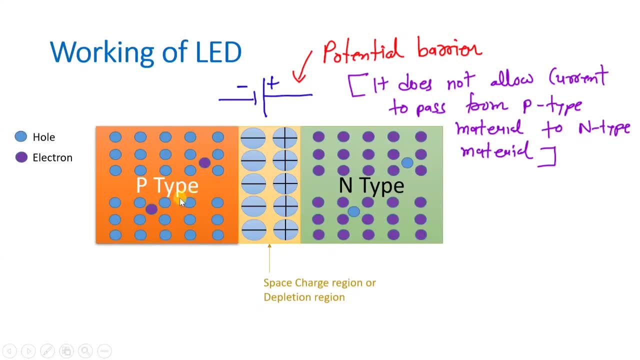 light emitting diode in forward wires you will have to apply greater voltage than the potential barrier voltage. then only there can be a conduction of current from p-type material to n-type material. now let us try to one understand how this LED functions. so to understand functioning, first we need to 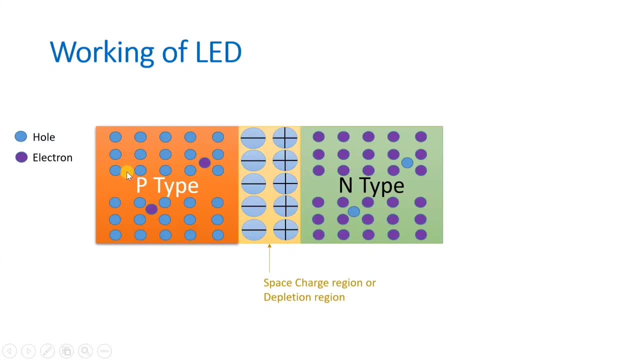 connect this LED in forward wires and to have forward wires connection, p-type material should be connected with positive terminal of battery and n-type material should be connected with negative terminal of battery and when you do this, holes of p-type material will jump over this side and electrons. 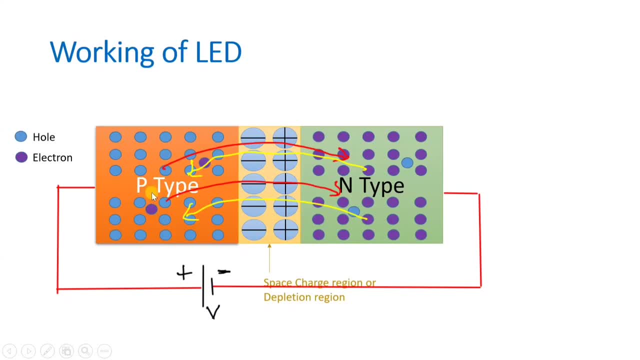 of n-type material will jump over this side and they will get recombined. and they recombines. you'll be finding they will be releasing energy as a light. now how that happens, you can observe: p-type material is having holes as a free charge carrier and n-type material is having electrons as a free charge. 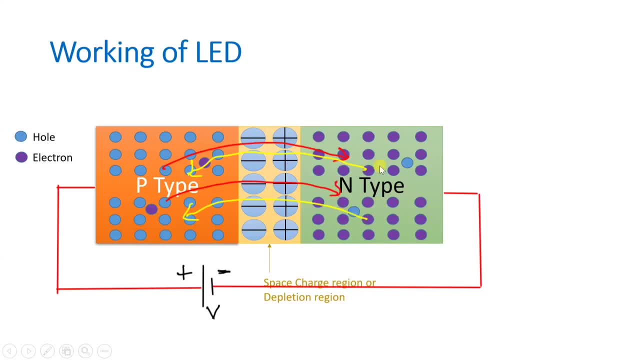 carrier and, as it is free charge carriers, those charge carriers will be there in conduction band. now those charge carriers are jumping from n-type to p-type and p-type to n-type. holes are jumping from p-type to n-type and it is getting combined with n-type. 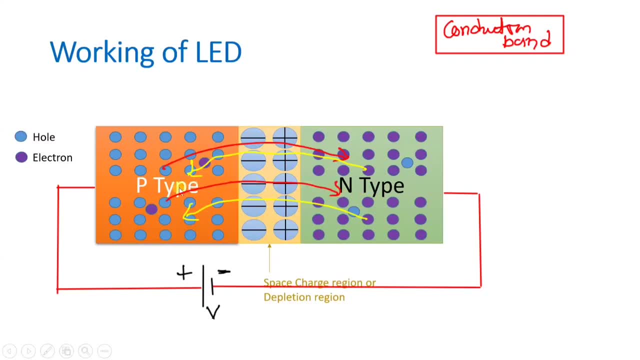 and electrons of n-type is jumping towards p-type material and it is getting combined with holes of p-type. so when that happens, so those free charge carriers will jump from conduction band to valence band and as it is jumping from conduction band to valence band, there will be a release of. 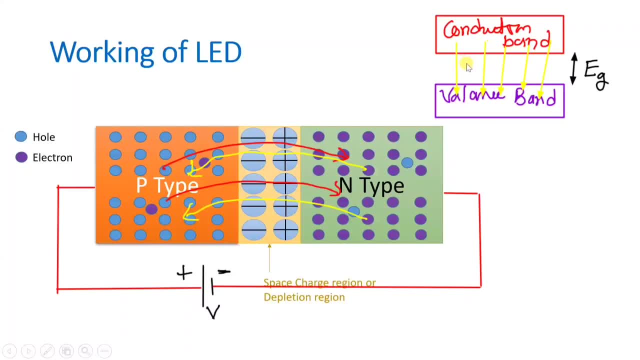 energy. let us say that energy is EG and that energy EG is equals to H into F, where H is playing constant and F is frequency of that transition and that frequency is C by lambda. so this energy, that is H into C by lambda, now see if this lambda 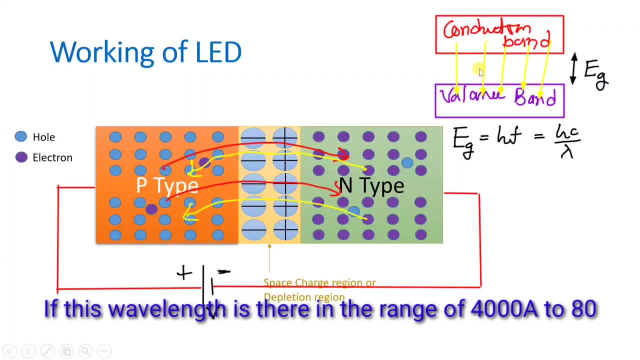 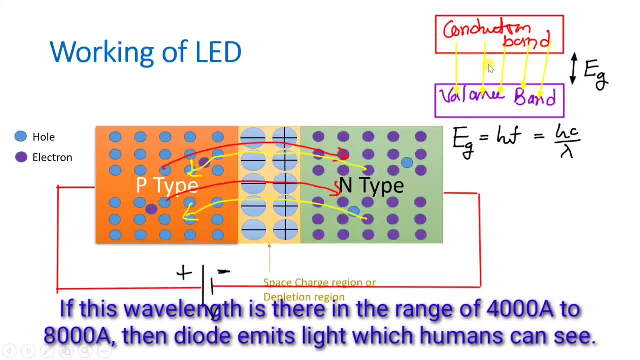 wavelength is staying in the vicinity of 4000 to an 8000 angstrom, then that release of energy will be energy of light signal, as human can see light with different colors and those colors are there in the vicinity of 4000 angstrom to 8000 angstrom. so when this release of energy 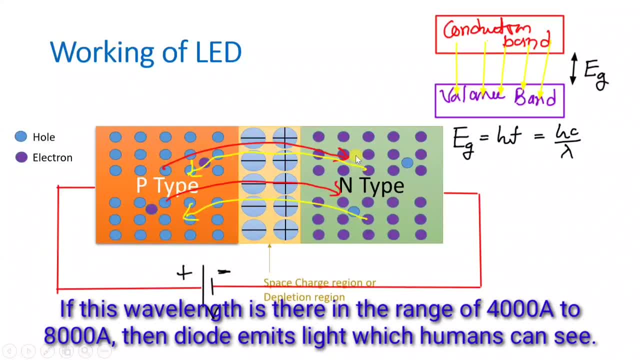 is happening, that release of energy should be there in the vicinity of 4000 strong to 8000 angstrom to see that as light. and here in LED we have such material which we use it as p-type and n-type material that gives that transition of. 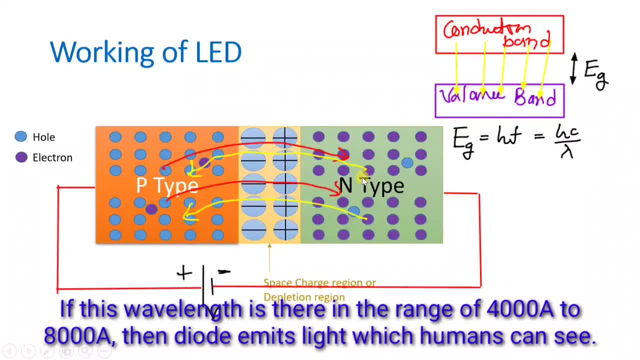 free charge carrier lies with the wavelength in between 4000 to 8000 angstrom. if that wavelength is beyond 4000 to 8000 angstrom, then humans cannot see light in theory. the wavelength is beyond 4000 to 8000, then humans cannot see light in theory. 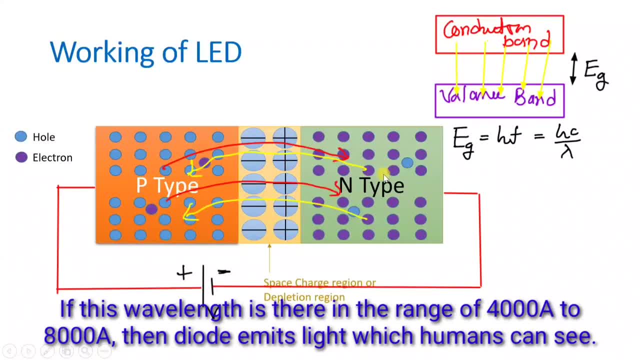 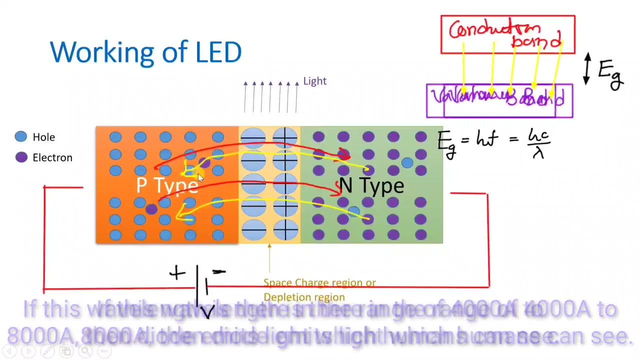 light and in normal pn junction diode you will be observing same process is happening, but as that wavelength is not there in the vicinity of 4000 angstrom to 8000 angstrom, it does not radiate light. so light will get emitted over here as if it is connected in forward bias. 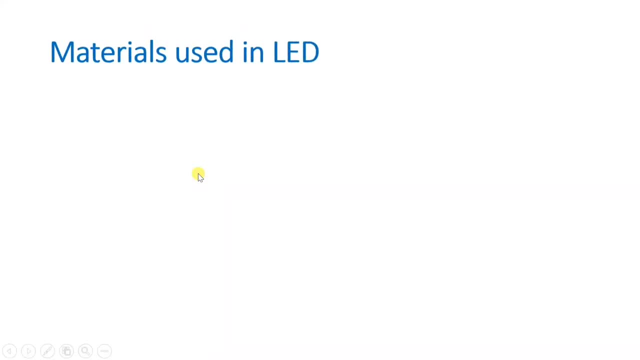 now there are some materials which we use it in led- gallium arsenide, that we use it to have infrared led, and you will be observing this type of material, gallium arsenide- that is to make infrared led, and we use that in the remote controls. so there are different types of remote control that you might be using nowadays, like tv remote. 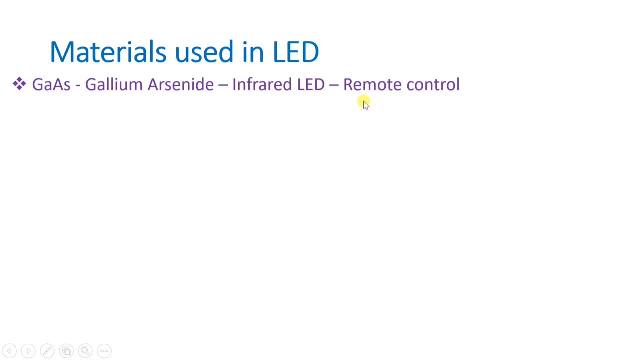 control, aclpc remote control. so in that led will be made up of gallium arsenide and that led is infrared led- gallium phosphide- that is even a very popular material which people are using it to form red or green color led- and gallium arsenide phosphide- that is what we are using it to have.